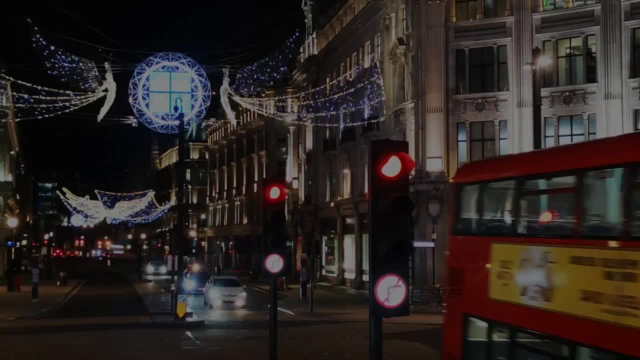 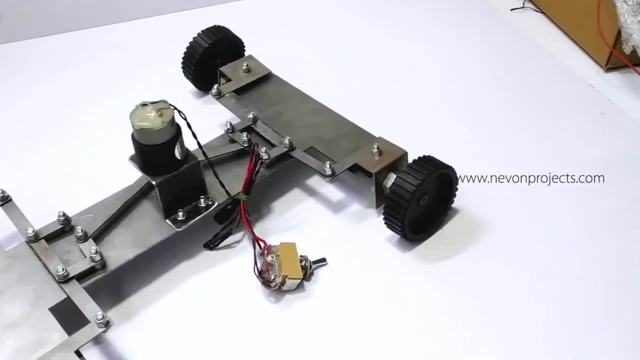 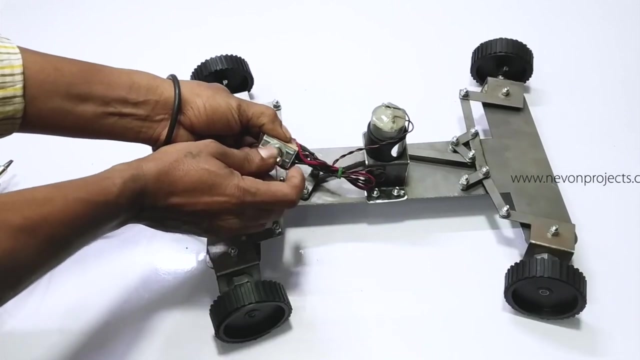 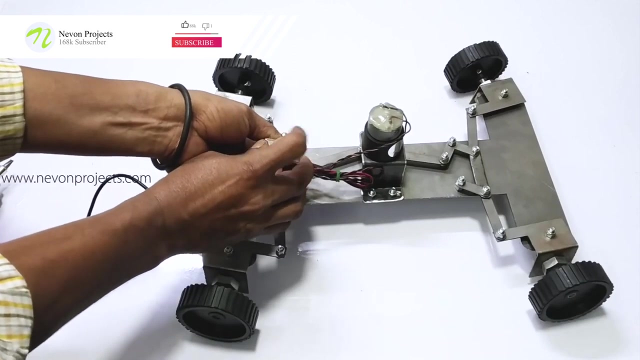 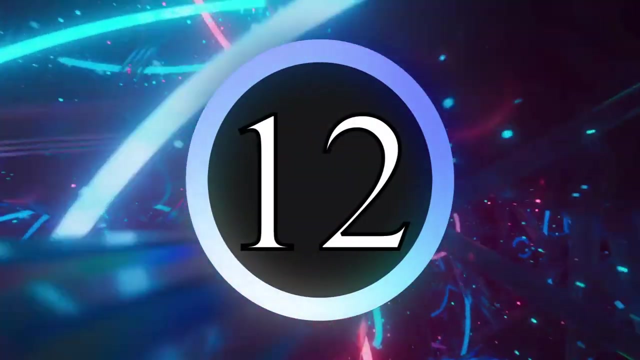 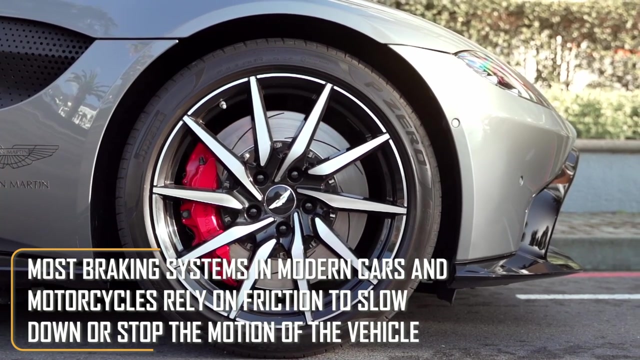 to assist in reducing the turning radius of the vehicle. This system uses motors to steer the vehicle's rear wheels along with the front ones, thereby enabling the vehicle to turn faster as well as more efficiently. Most braking systems in modern cars and motorcycles rely on friction to slow down or stop the motion of the vehicle. 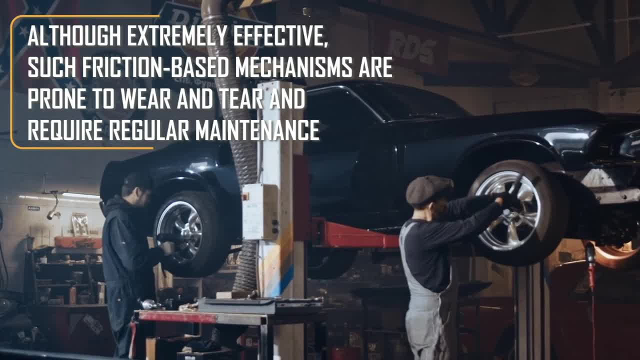 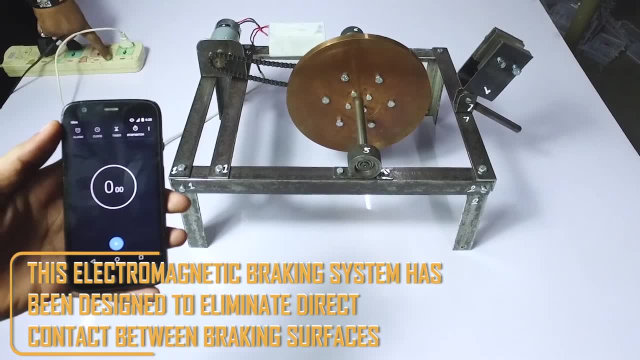 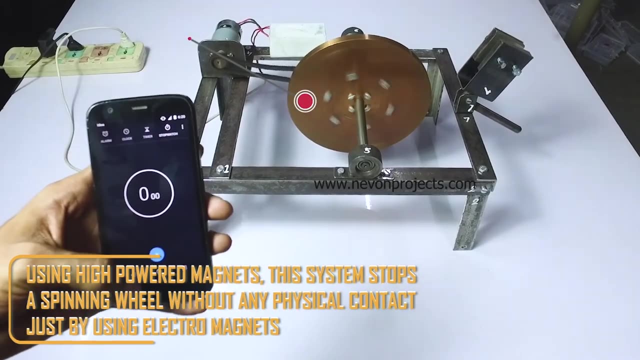 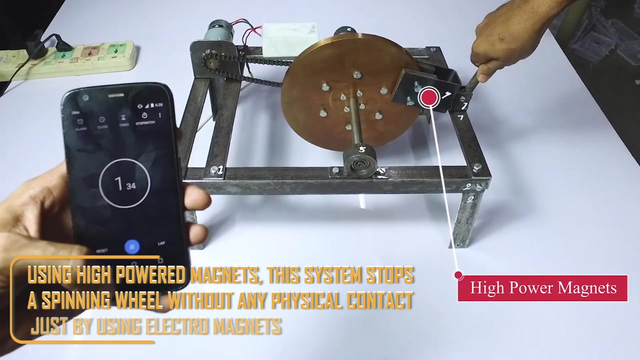 Although extremely effective, such friction-based mechanisms are prone to wear and tear and require regular maintenance. This electromagnetic braking system has been designed to eliminate direct contact between the brake and the surface of the wheel Using high-powered electromagnets. this system stops a spinning wheel without any physical contact, just by using electromagnets. 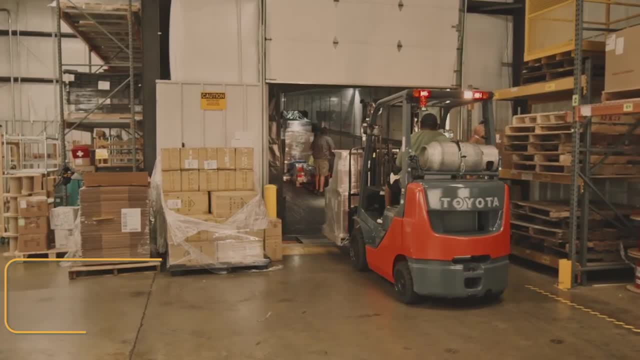 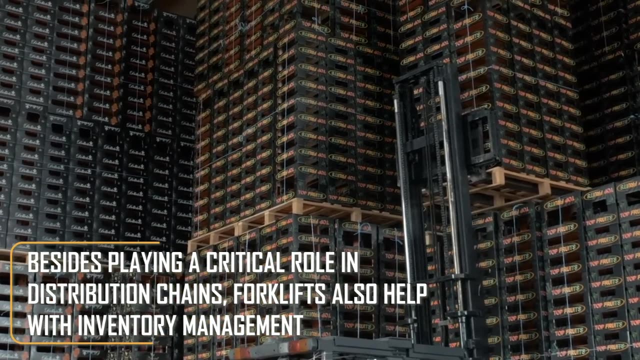 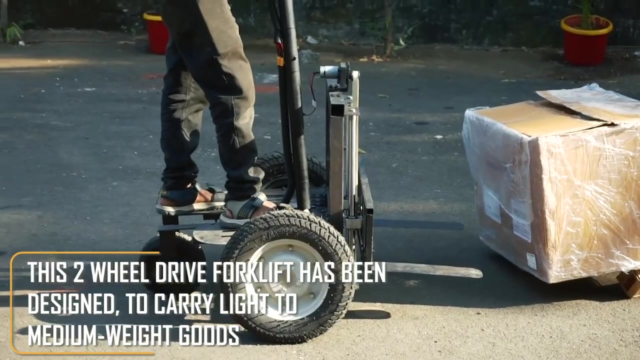 Two-wheel drive forklift. Forklifts are an irreplaceable aspect of warehouses and go-downs. Besides playing a critical role in distribution changes, forklifts also help with inventory management. This two-wheel drive forklift has been designed to carry out medium to lightweight goods. 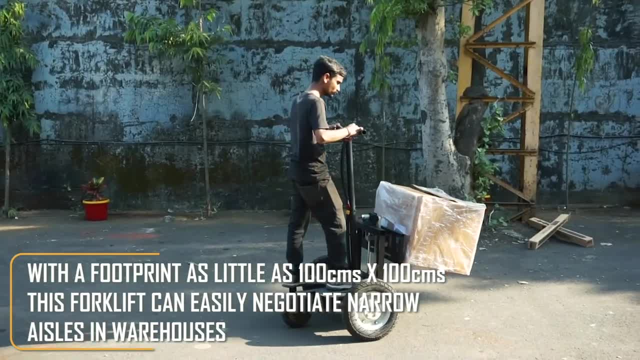 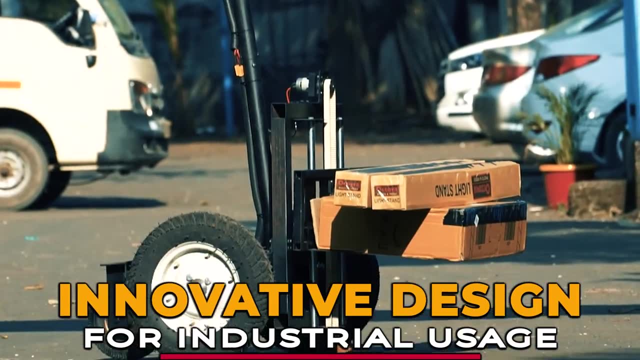 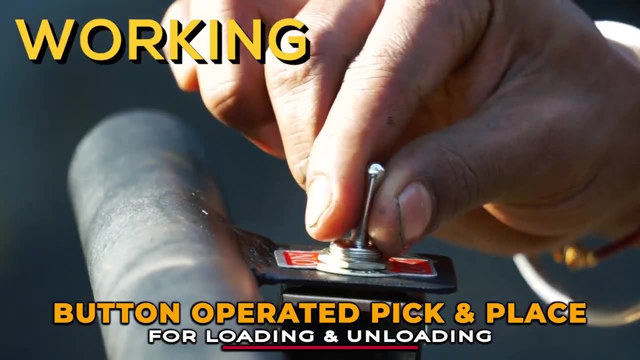 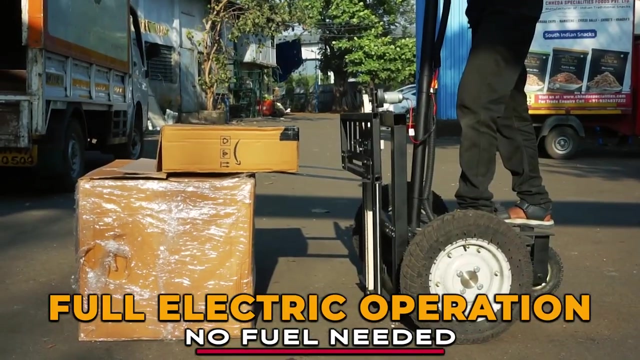 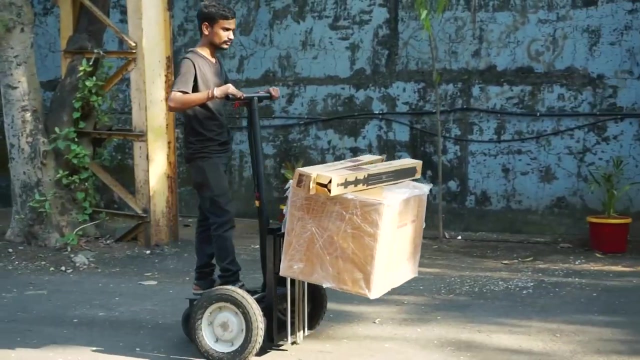 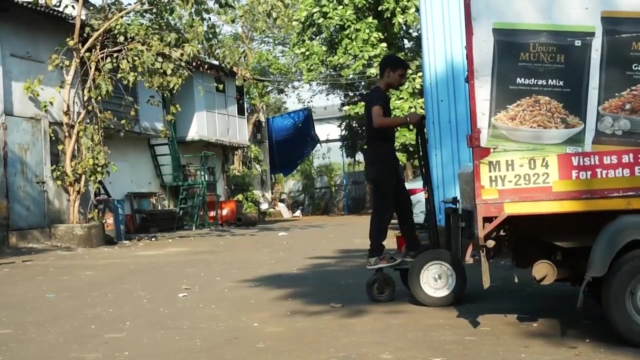 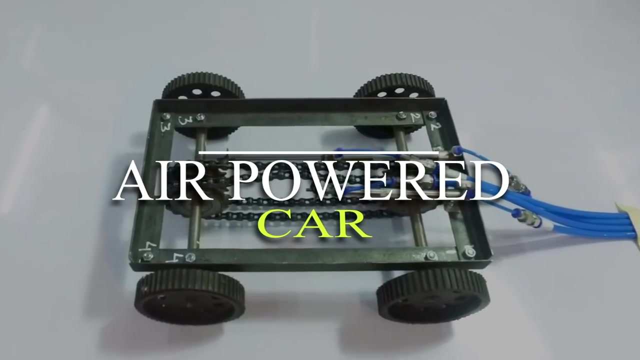 With a footprint of as little as 100 x 100 cm, this forklift can easily negotiate narrow aisles in the warehouse. It acts as a wind-shrinkable box city. This iswasser resistant, a preferable secondka station. Air powered car. 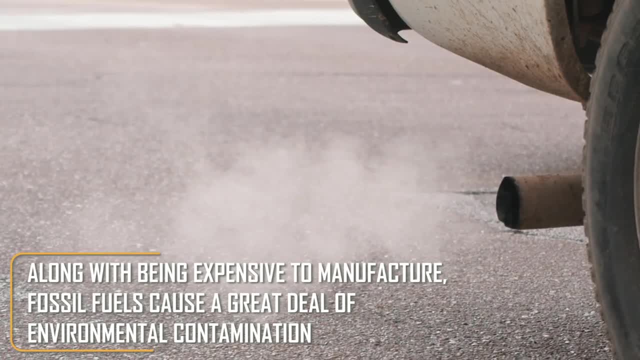 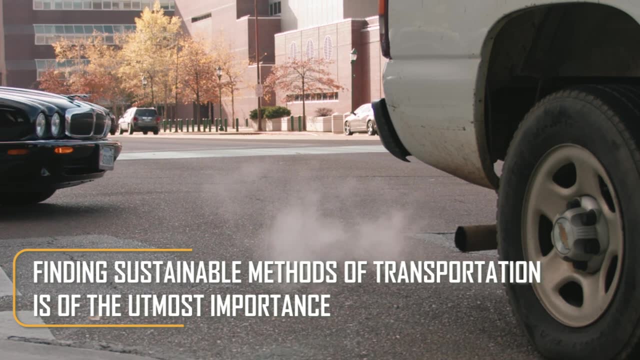 Willy Dec Adelasin. Along with being expensive to manufacture, Willy Dec Adelasin, fossil fuels can cause a great deal of environmental contamination. Finding suitable methods of transportation is of utmost importance. This air-powered car is powered by a pair of pneumatic pistons. 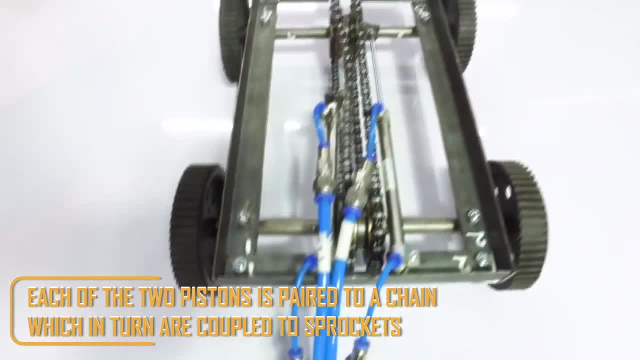 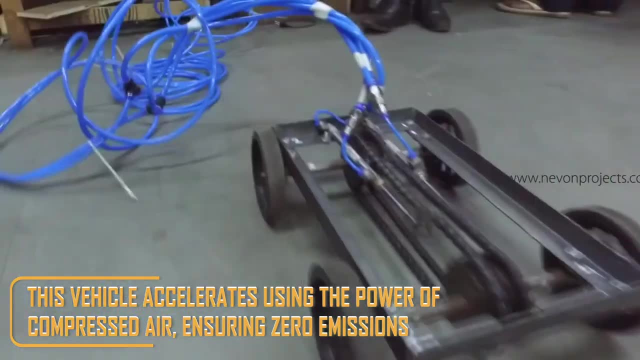 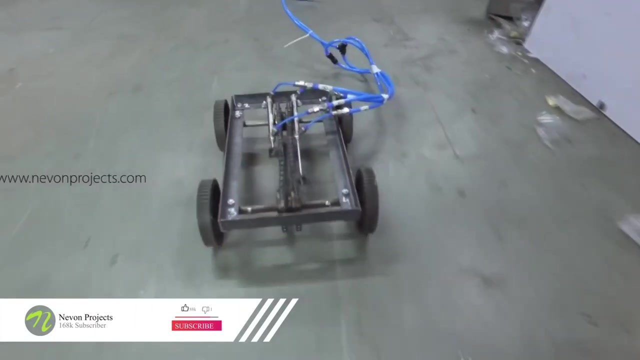 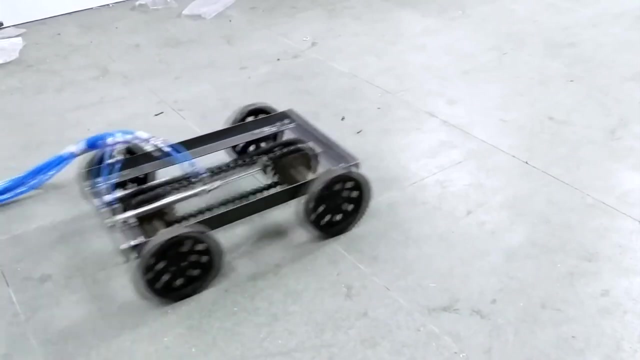 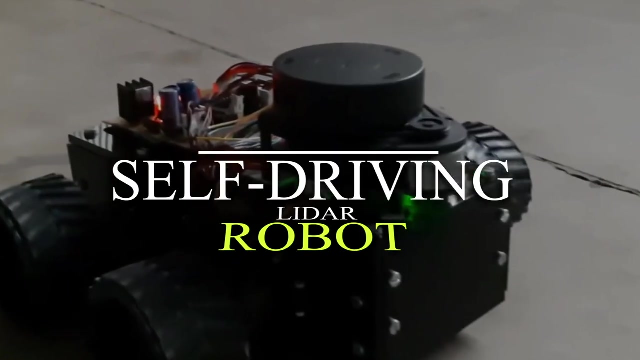 Each of the two pistons is paired to a chain, which in turn are coupled to sprockets, So this vehicle accelerates using the power of compressed air, ensuring zero emissions. Self-Driving LiDAR Robot. We have reached the era of electric cars. 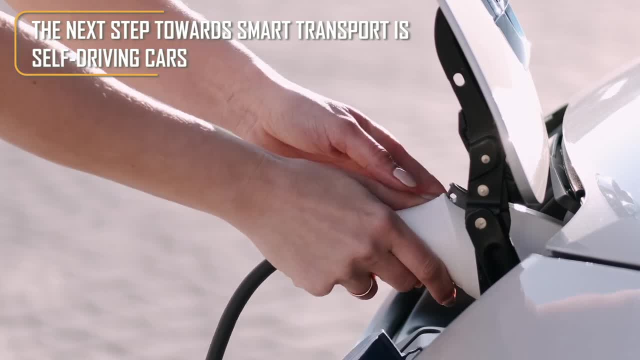 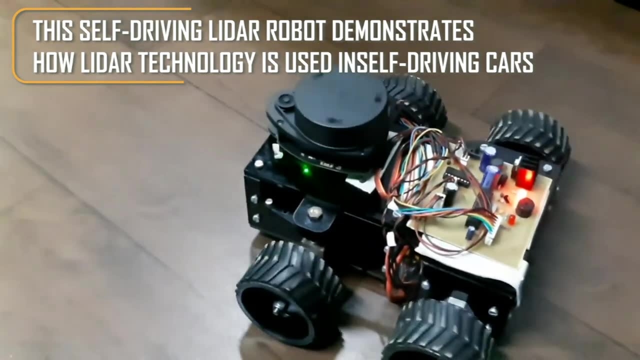 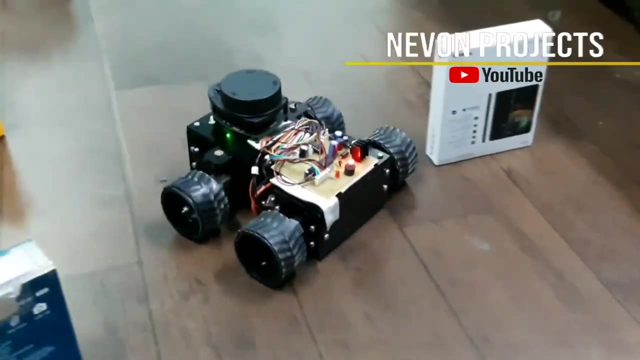 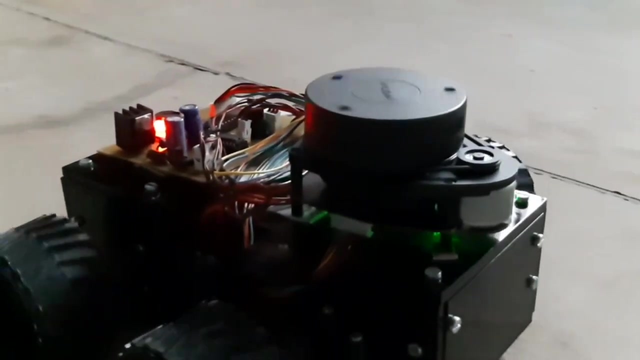 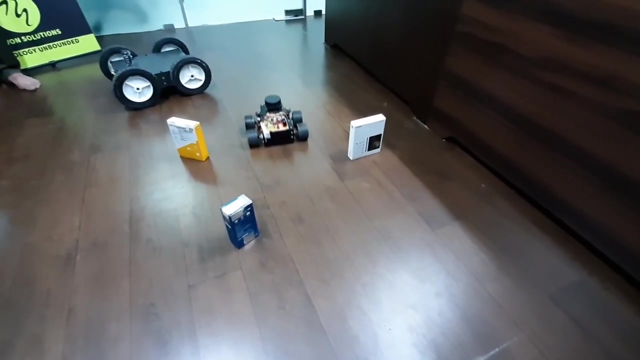 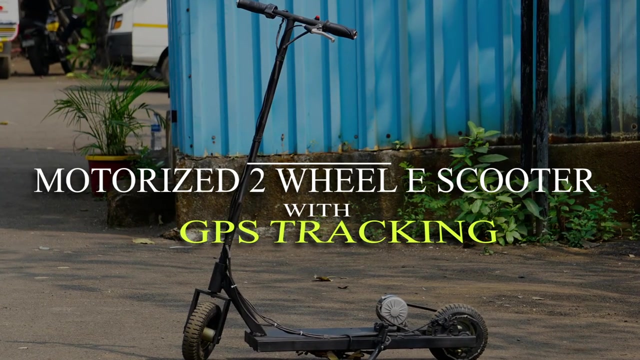 The next step towards smart transportation is self-driving cars. This self-driving LiDAR robot demonstrates how the LiDAR technology is used in self-driving cars. How to become a smart learner: Never give up. Motorized Two Wheel e-scooter with GPS Tracking. 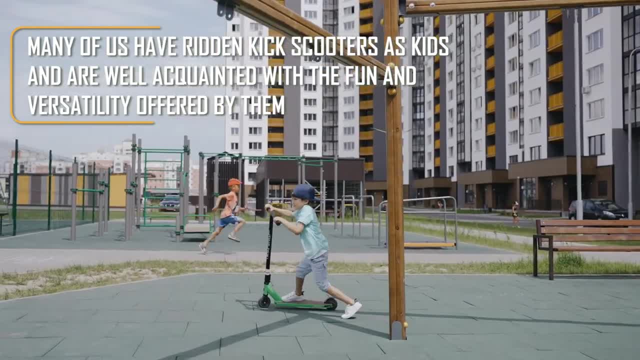 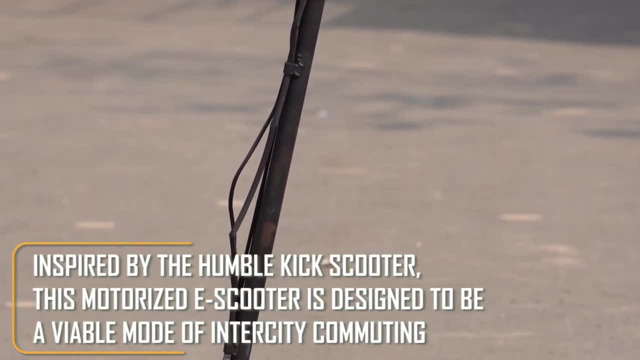 Many of us have ridden the kick scooters as kids and we are well acquainted with the fun and versatility offered by them. Inspired by the humble Kick Scooter, this motorized e-scooter is designed to be a viable mode of intercity commuting. 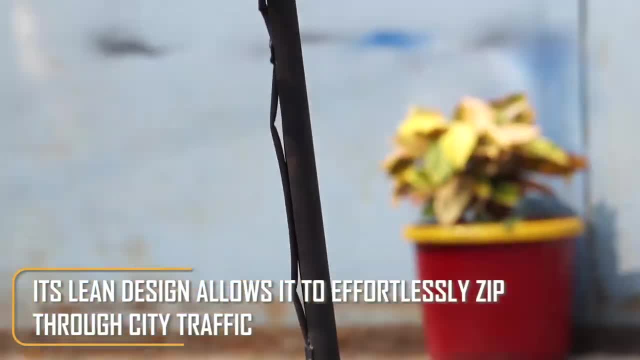 This might be the case with the Alpine varios. The new motorized e-scooter has been brought to the fore by the Ford Group of India for about 7 years, allows it to effortlessly zip through the city traffic Using an electric motor mated to a belt drive. 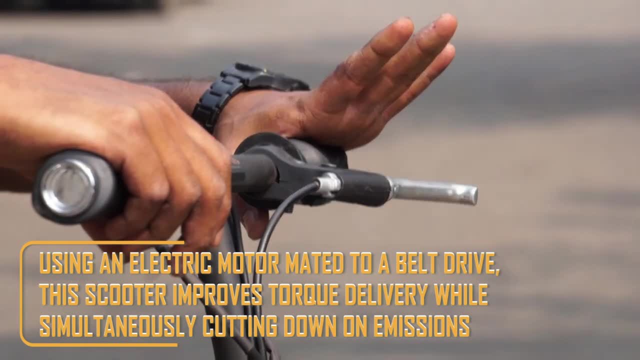 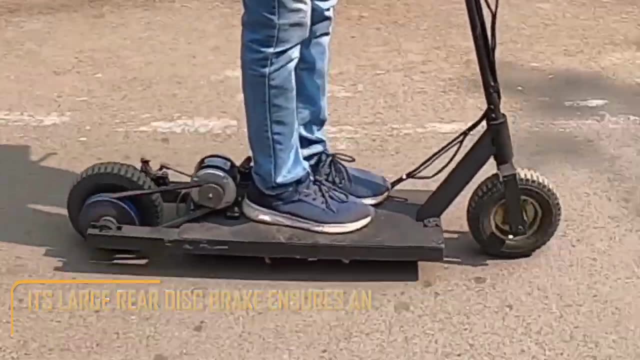 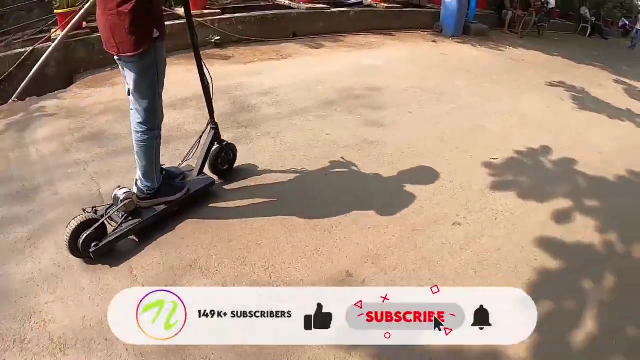 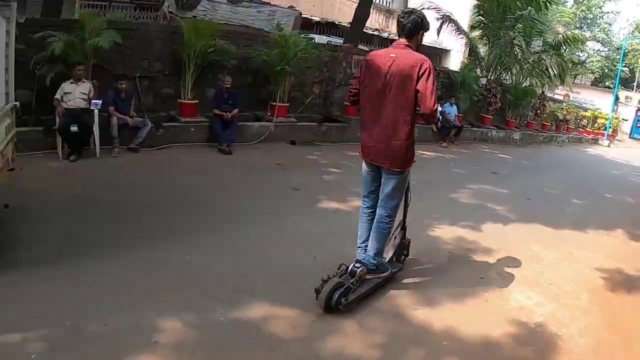 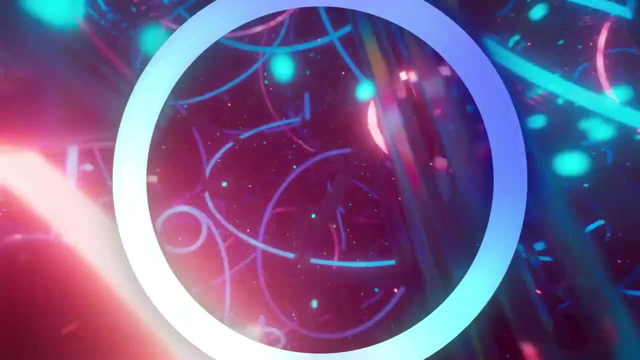 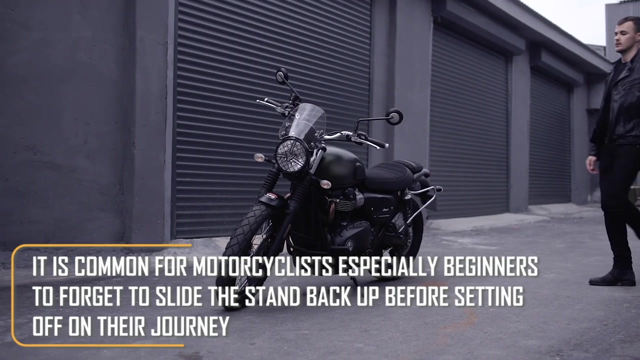 this scooter improves torque delivery while simultaneously cutting down on emissions. Its rare disc brake ensures an extremely short stopping distance, and this system has also been equipped with a GPS tracking system. Smart Bike Stand: It is common for motorcyclists, especially beginners, to forget to slide the stand back up. 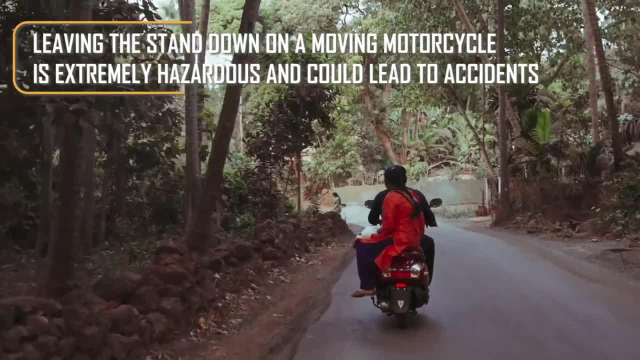 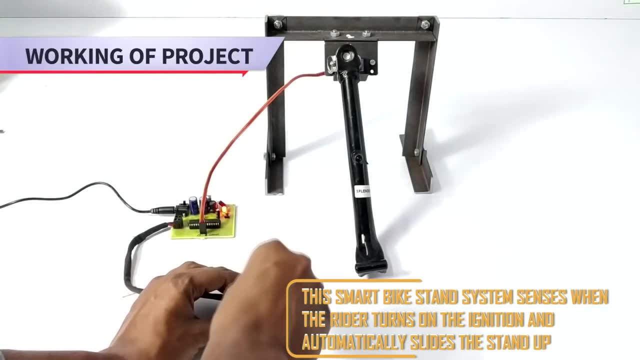 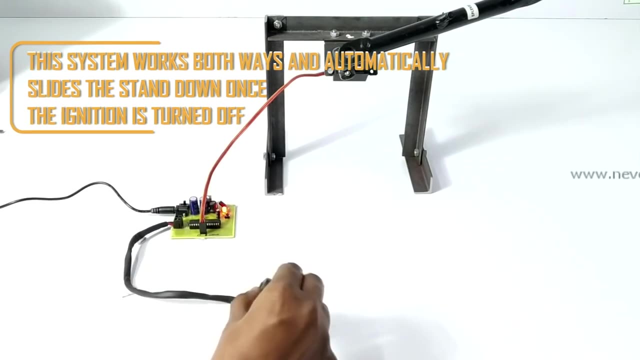 before setting off on their journey. Leaving the stand down on a moving motorcycle is extremely hazardous and could lead to accidents. This smart bike stand system senses when a rider turns on the ignition and automatically slides the stand up. This system also works both ways and automatically slides the stand down. 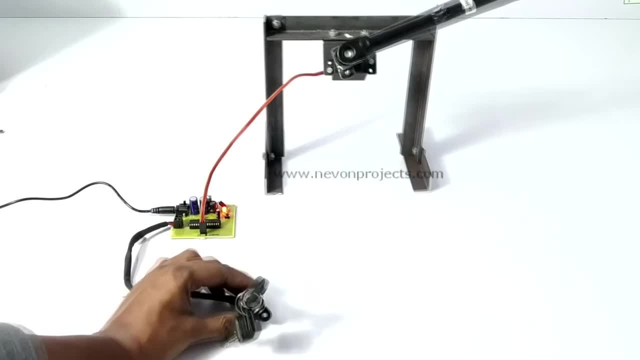 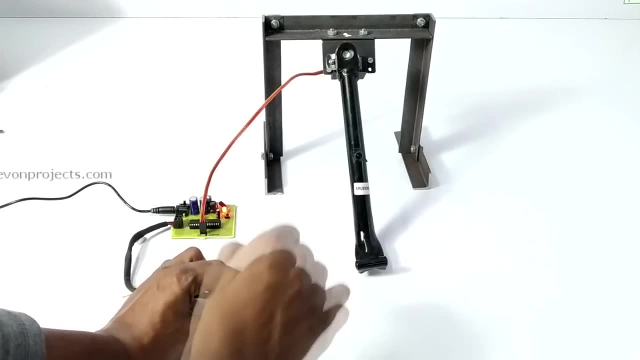 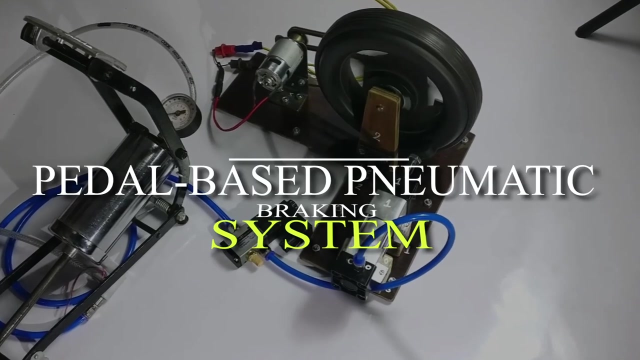 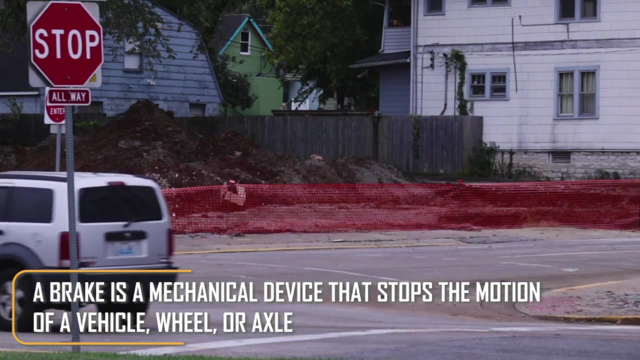 once the ignition is turned off. Pedal-Based Pneumatic Braking System. Pedal-Based Pneumatic Braking System. Pedal-Based Pneumatic Braking System. A brake is a mechanical device that stops the motion of a vehicle, wheel or an axle. 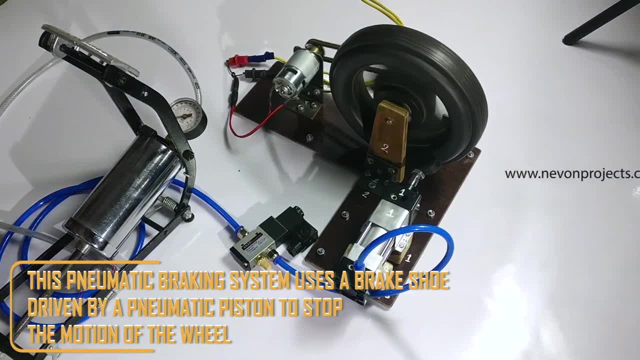 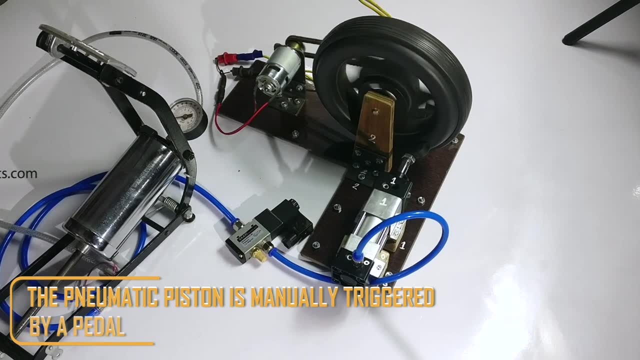 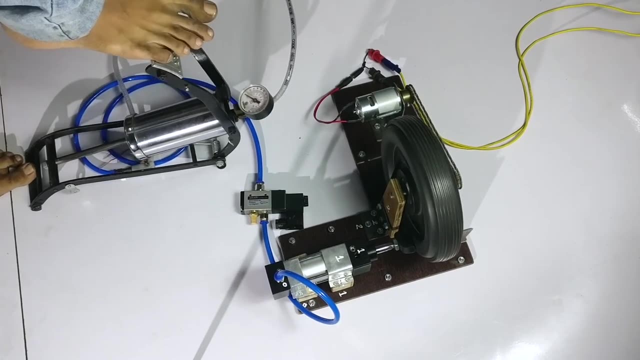 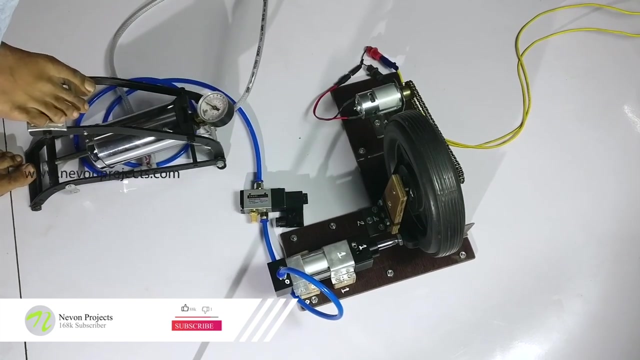 This pneumatic braking system uses a brake shoe driven by a pneumatic piston to stop the motion of a wheel. This pneumatic piston is manually triggered by a pedal. Pedal-Based Pneumatic Braking System. Pedal-Based Pneumatic Braking System. 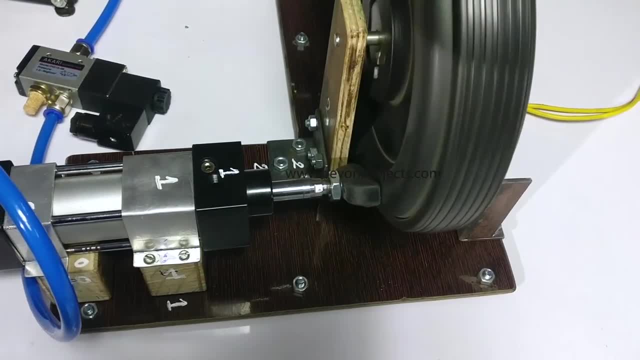 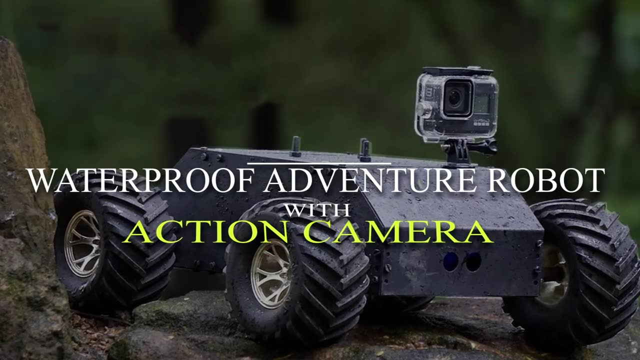 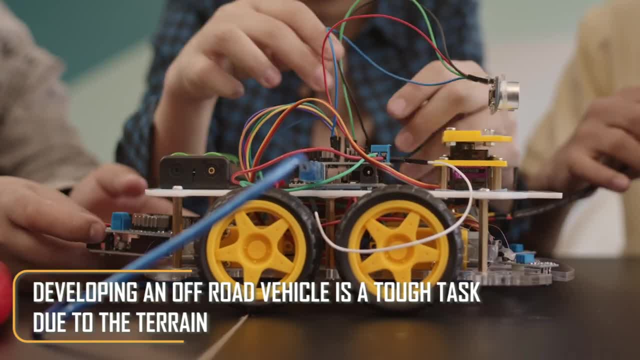 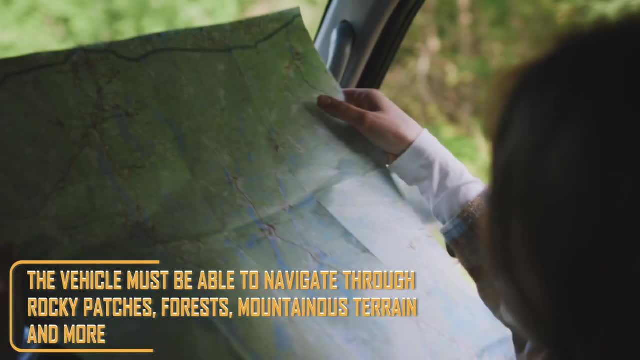 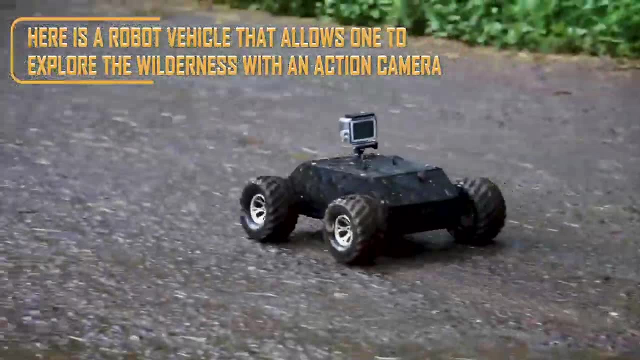 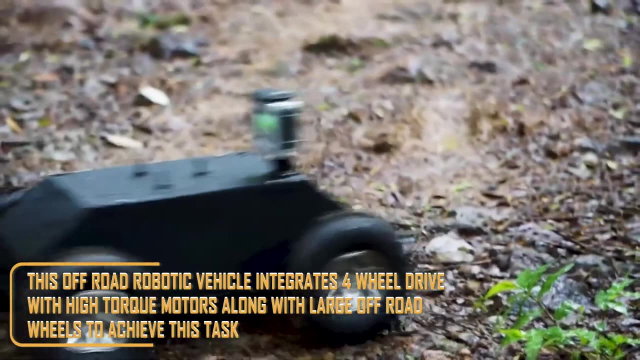 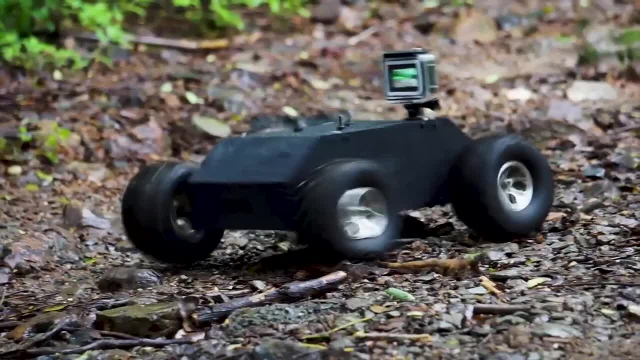 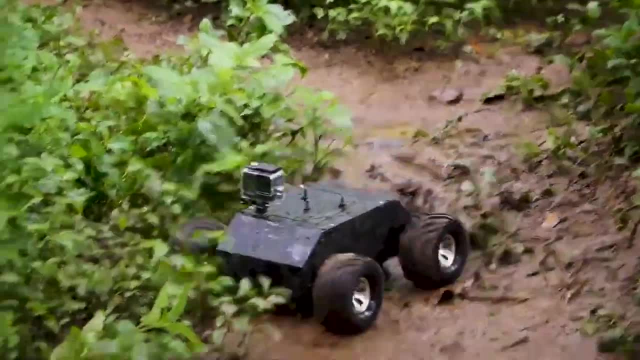 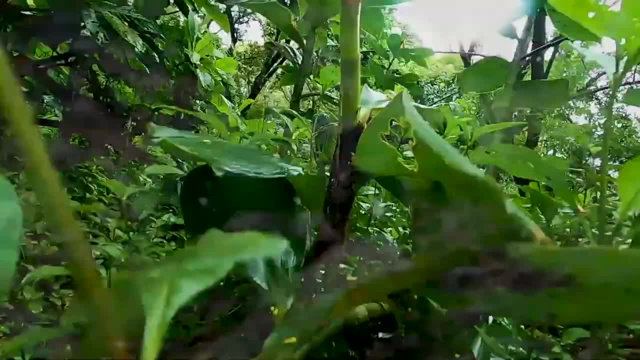 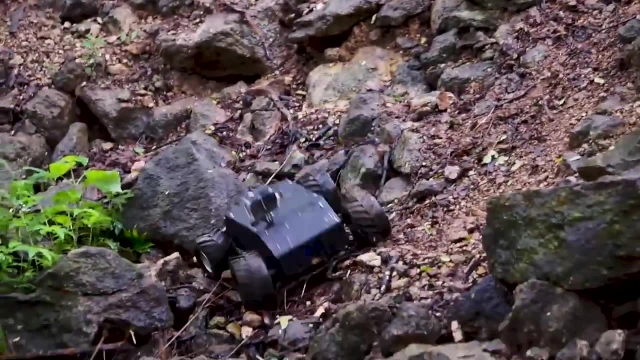 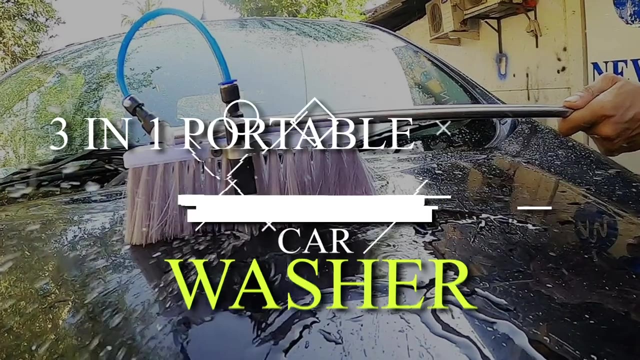 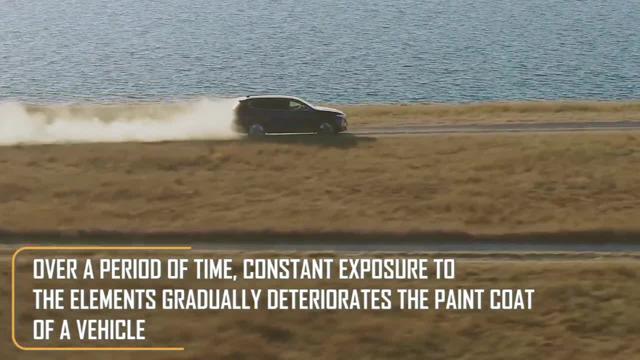 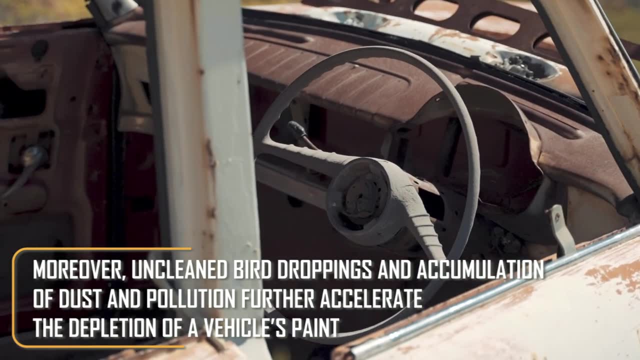 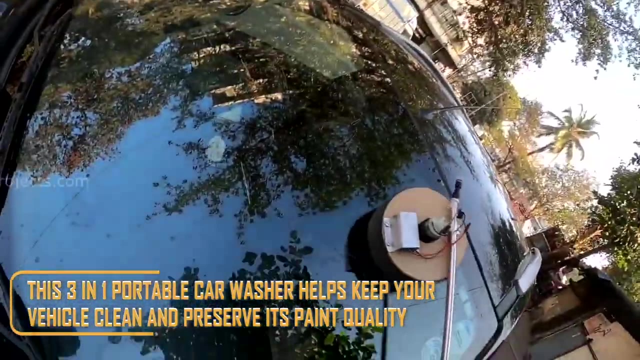 the elements gradually deteriorates the paint coat of a vehicle. Moreover, unclean bird droppings and accumulation of dust and pollution further accelerate the depletion of a vehicle's paint. This 3-in-1 car washer helps keep your vehicle clean and preserve its paint quality. 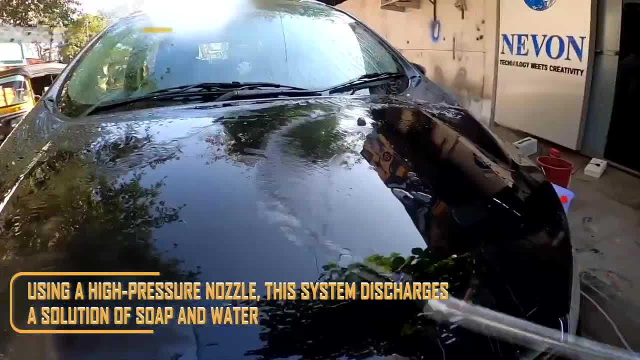 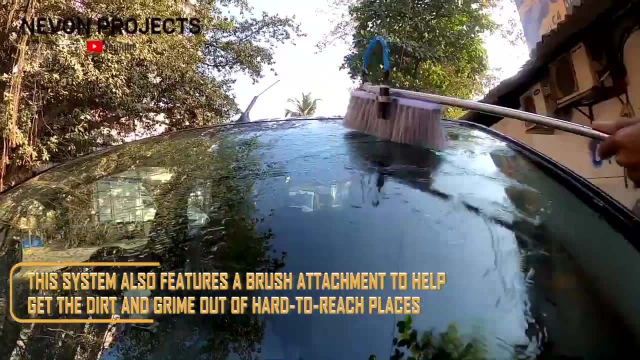 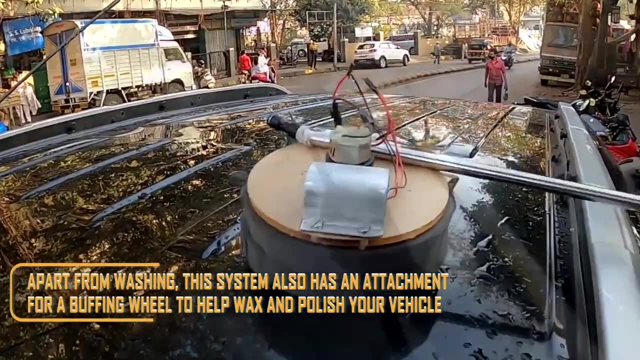 Using a high-pressured nozzle, this system discharges a solution of soap and water. This system also features a brush attachment to help get the dirt and grime out of hard-to-reach places. Apart from washing, this system also has an attachment for a buffing wheel to help wax. 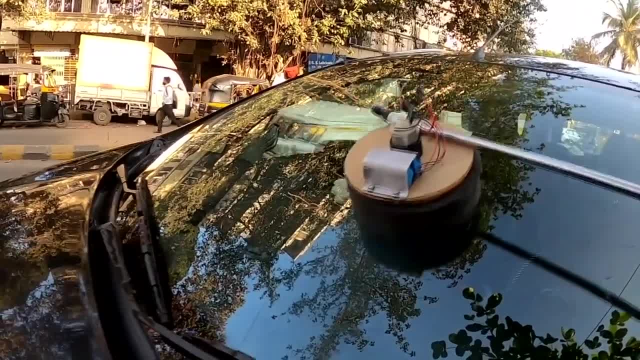 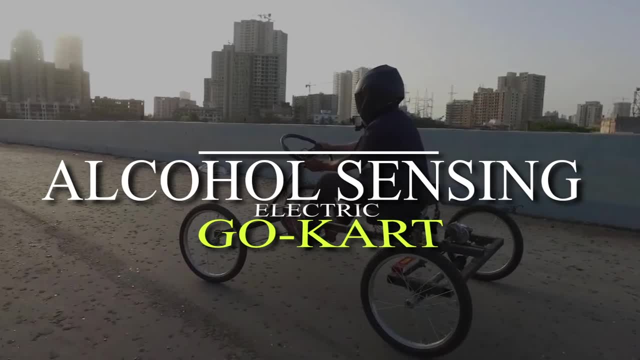 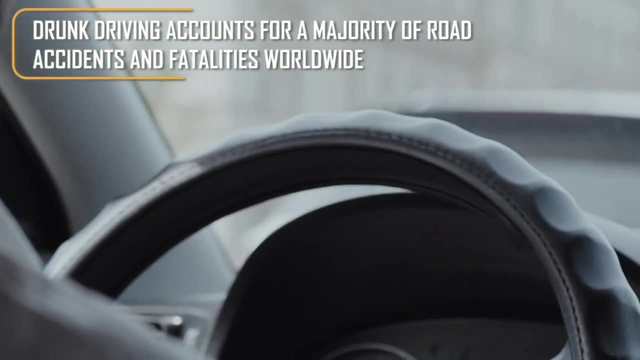 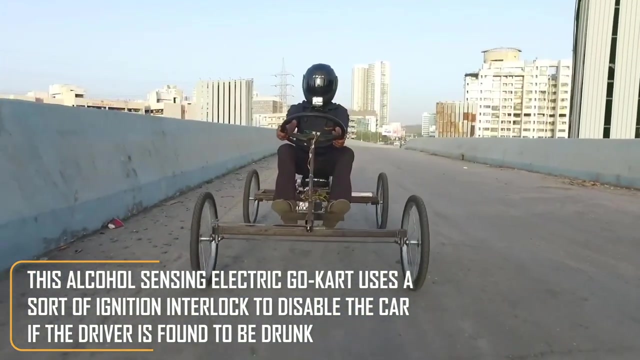 and polish your vehicle. 4-Alcohol Sensing Electric Go-Kart. Drunk driving accounts for a majority of road accidents and fatalities worldwide. This alcohol-sensing electric go-kart uses a sort of ignition interlock to disable the car if the driver is found to be drunk. 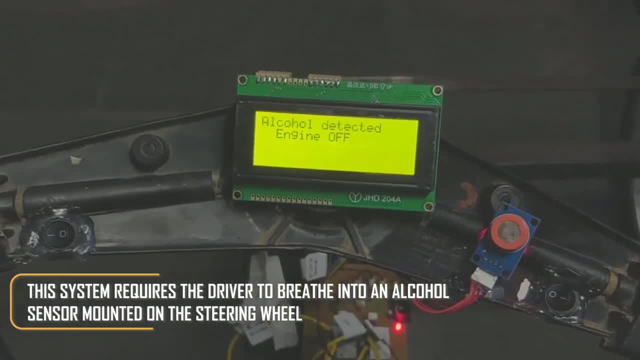 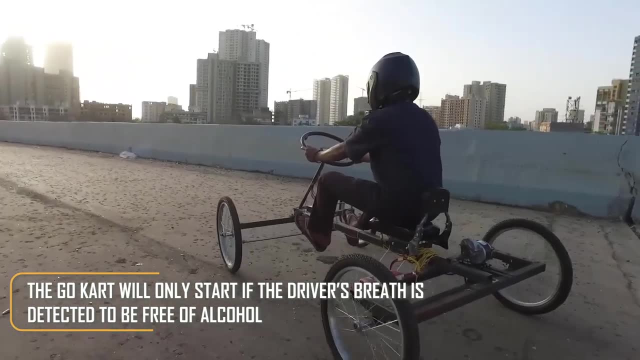 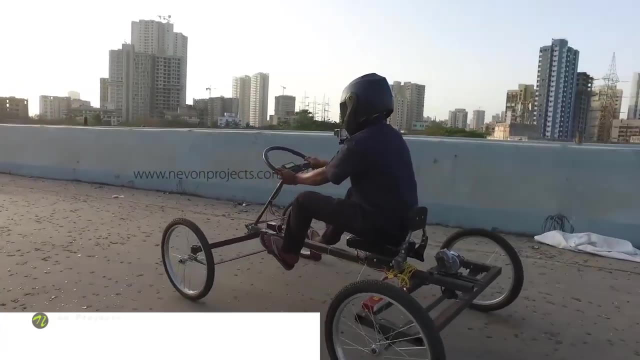 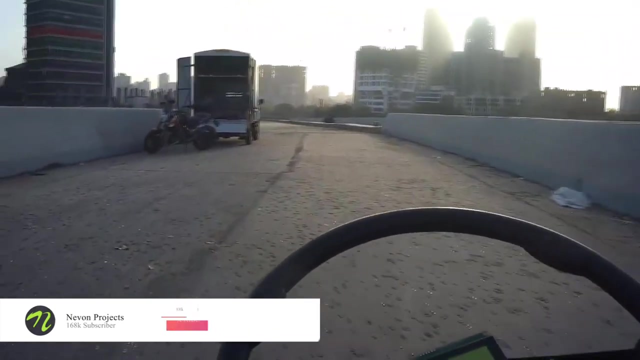 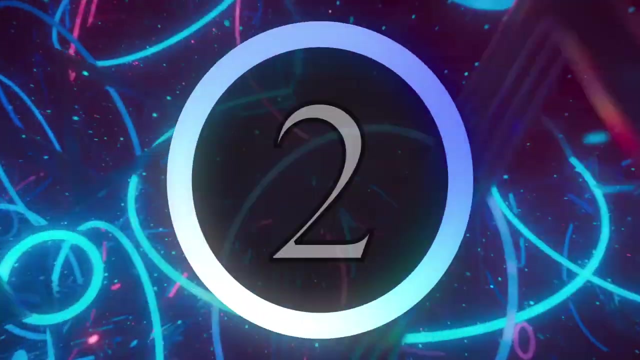 This system requires the driver to breathe into an alcohol sensor mounted on the steering wheel. The go-kart will only start if the driver's breath is detected to be free of alcohol. 5-Intelligent Mechanic Braking System. 6-Intelligent Mechanic Braking System. 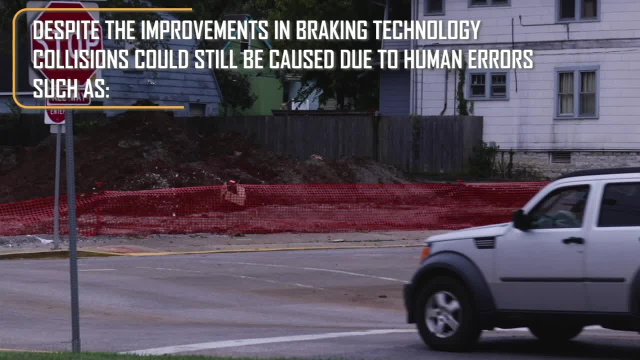 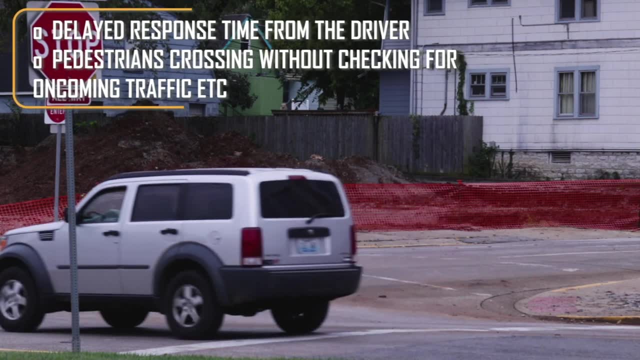 7-Intelligent Mechanic Braking System. 7-Intelligent Mechanic Braking System- braking system. Despite the improvements in braking technology, collisions could still be caused due to human errors, such as delayed response time from the driver, pedestrians crossing without checking. 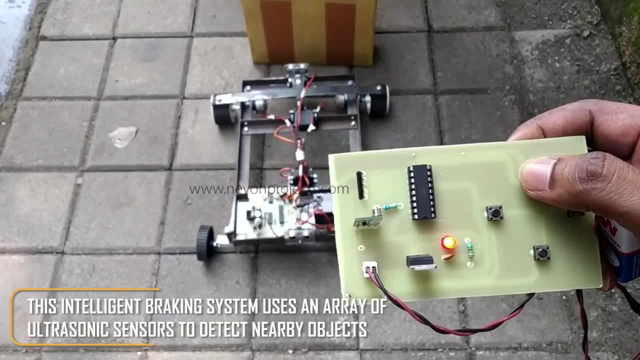 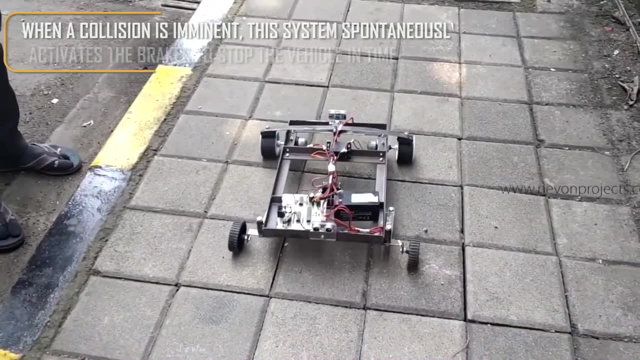 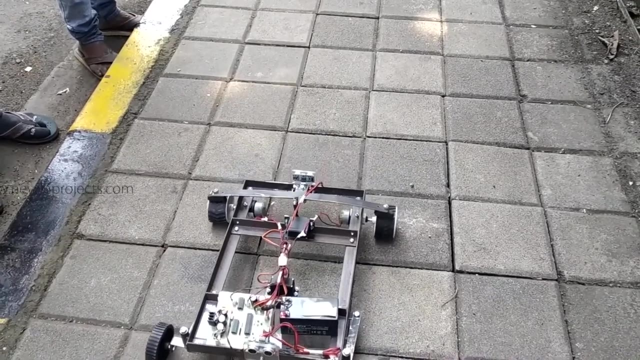 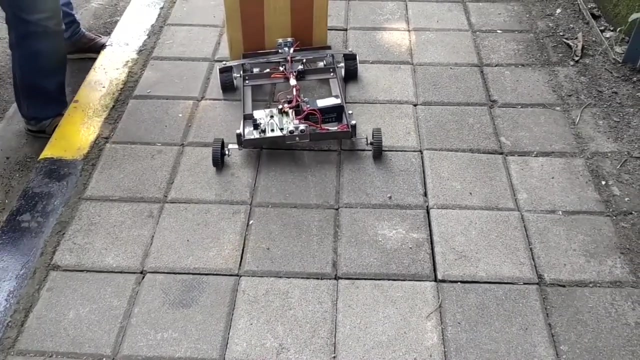 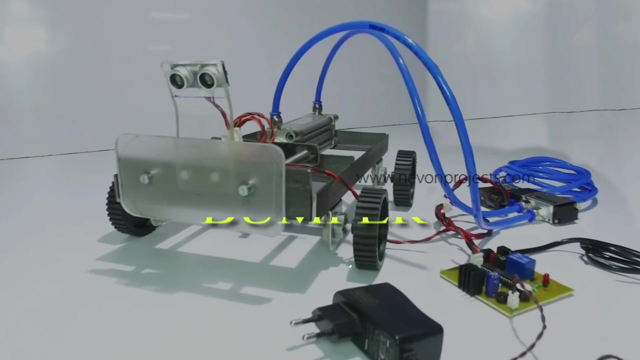 for oncoming traffic. This intelligent braking system uses an array of ultrasonic sensors to detect nearby objects. When collision is imminent, the system spontaneously activates the brakes to stop the vehicle in its time. Air Powered Pneumatic Bumper. In the event of a crash or a car bump, the bumper is supposed to bear the first brunt.